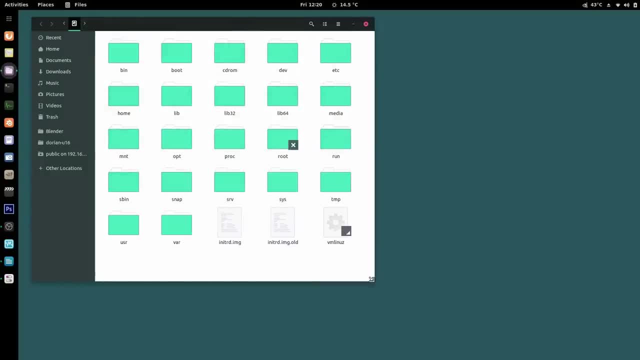 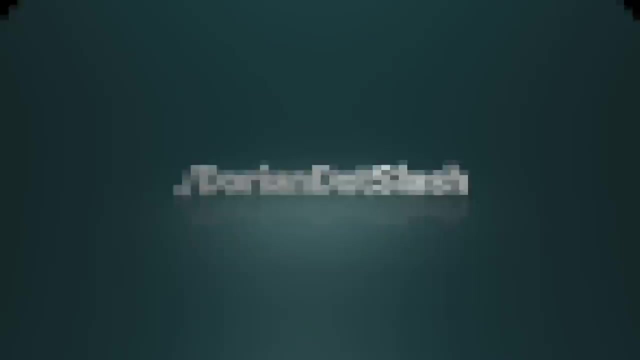 your videos? Same thing. That is until they explore up the tree looking for the C drive. Where's program files? Where's the directory that Linux is installed into? How do you find anything? Let me explain. I'll take a quick minute here for new Linux users coming from Windows. 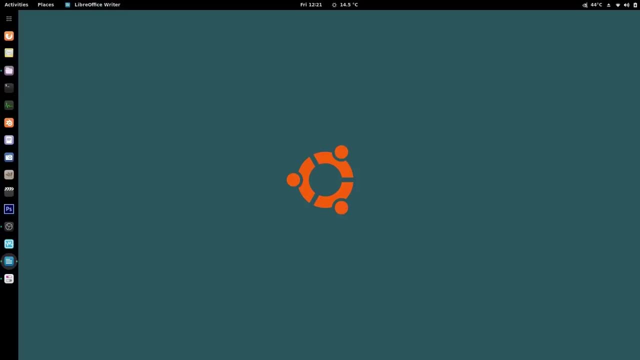 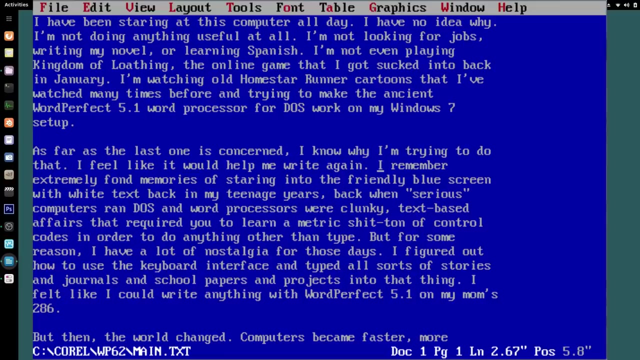 Windows and Linux evolved in very different ways. Once upon a time there was a thing called MS-DOS, the Disk Operating System. It was command line only, but you could still run programs, games and WordPerfect, but you didn't need Windows. 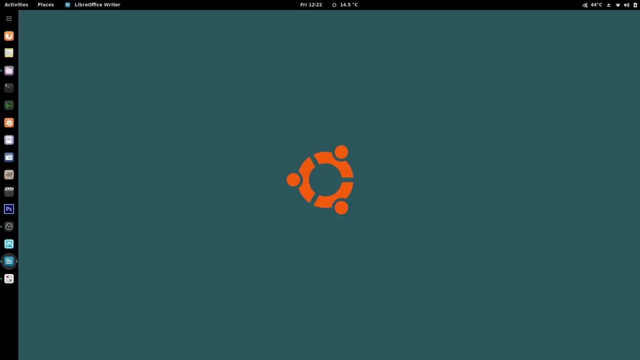 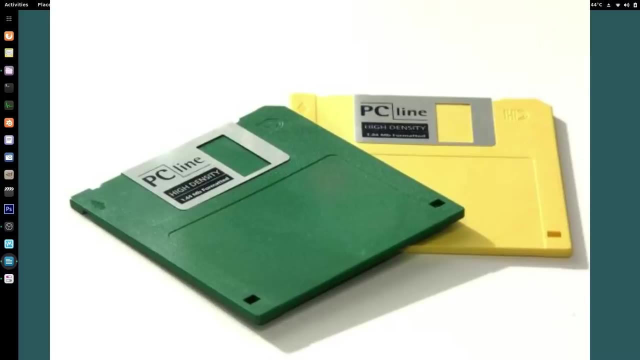 Windows was added to PCs and you could install it on top of DOS. You would start up your computer and type in win to start Windows. It used letters to assign drives, with A and B being removable disks, since early PCs only had floppy drives, With the addition of hard drives. 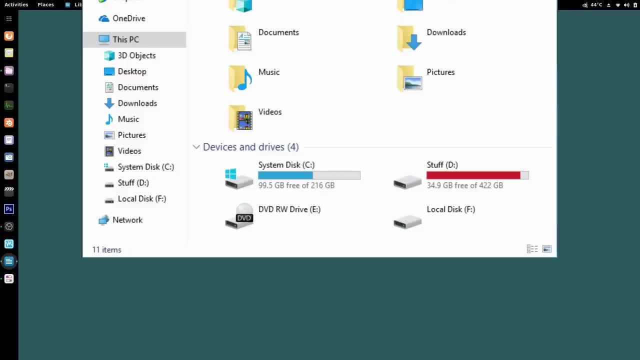 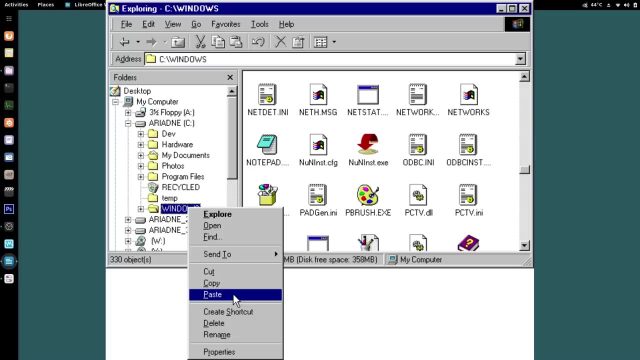 the letter C became the letter for your internal disk. Additional disks were given the next available letter. You could install things in DOS wherever you wanted to. Windows installed itself in its own directory, called, funny enough, Windows. Later Microsoft changed how it booted. 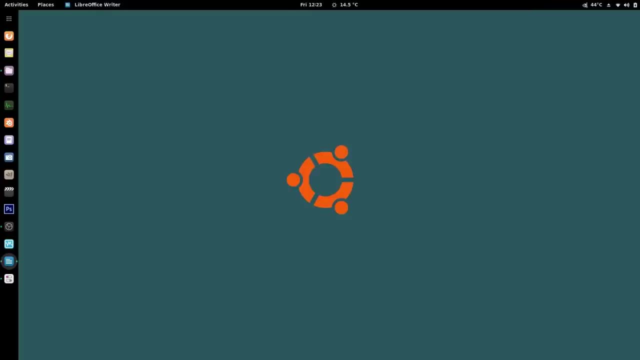 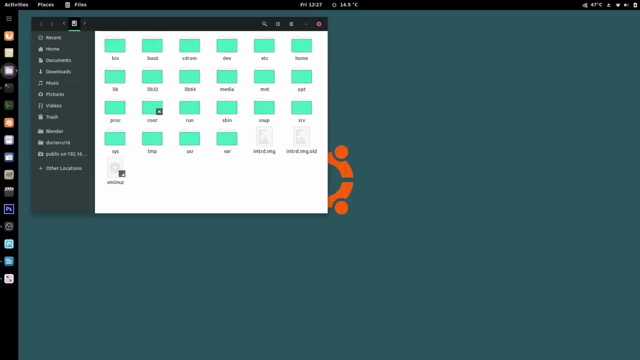 by evolving their kernel to be less and less dependent on DOS and eventually allowed Windows to boot directly without DOS at all. Microsoft's file directory structure kind of stayed the same. Now, Linux is different, and so is its file structure. It also doesn't. 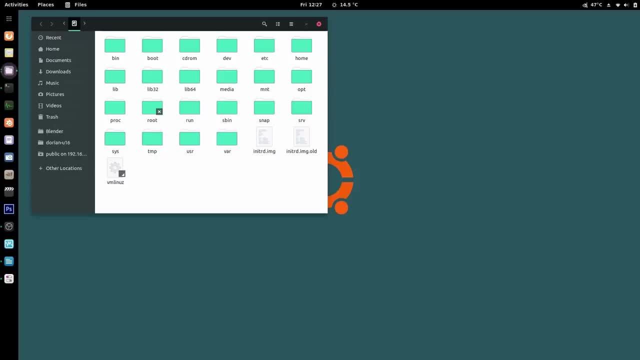 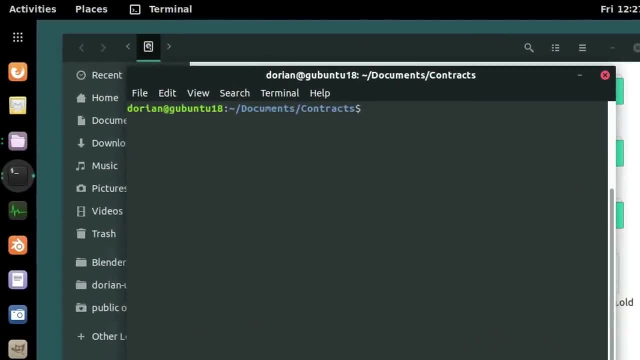 install applications, like Windows does. Starting with Windows 95,, Microsoft created the program files directory, which was the default installation directory for most applications. For the most part, Linux follows Unix traditions, which is why it uses the forward slash instead of the backslash. 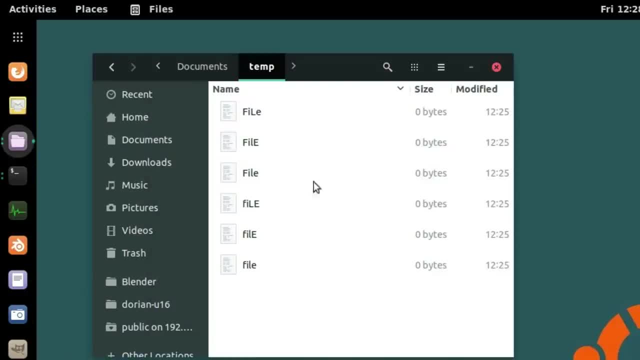 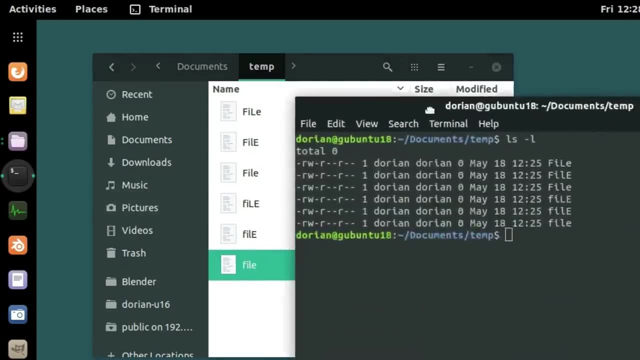 like Windows, Linux also cares about capitalization, so you can have things like this: File, file, file, file, file, file. As you can see, while they're all named file, they all use different capitalization, so Linux will allow this, because they're technically not. 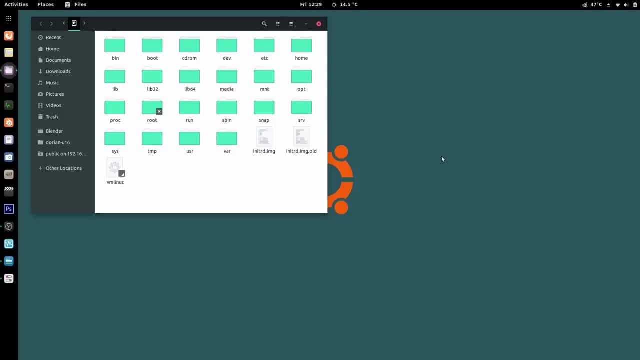 named exactly the same. Mac users who have explored their hard drives might find Linux a little more familiar. This is because Macs also evolved from a Unix ancestor, more specifically BSD. So let's have a look at the root and go over how all this works, This layout. 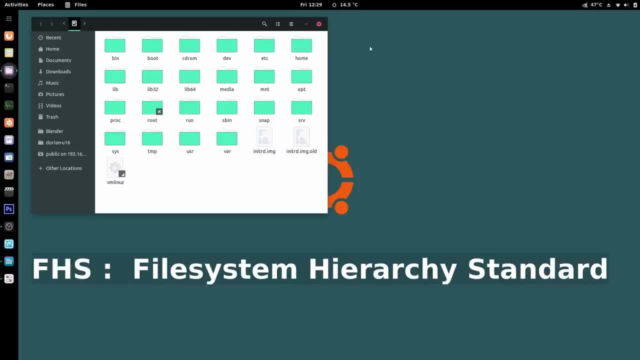 for the most part is outlined in the file system hierarchy standard, or FHS, which defines the structure and layout and is maintained by the Linux foundation. I want to note here that not all distributions follow this. Some do their own special thing. Also, several 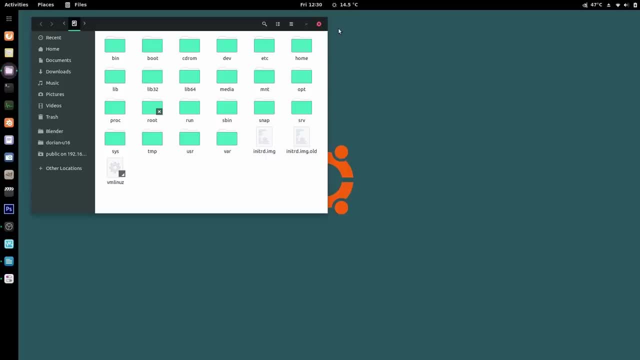 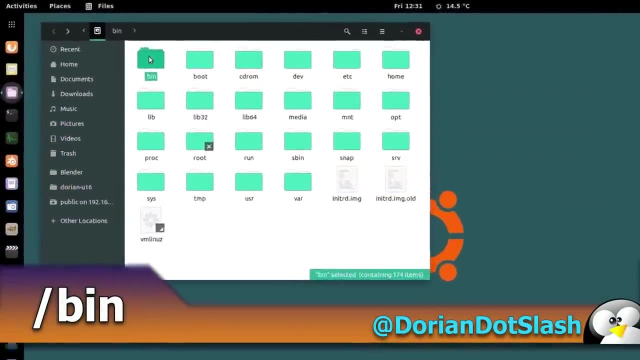 ways of structuring the folders has changed over the years, but most of what follows still applies in most cases. So let's go end to end, starting with bin Bin being short for binaries. These are the most basic binaries, which is another word for programs or applications, Things like 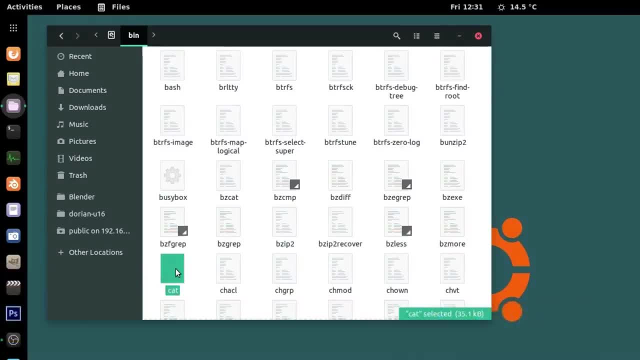 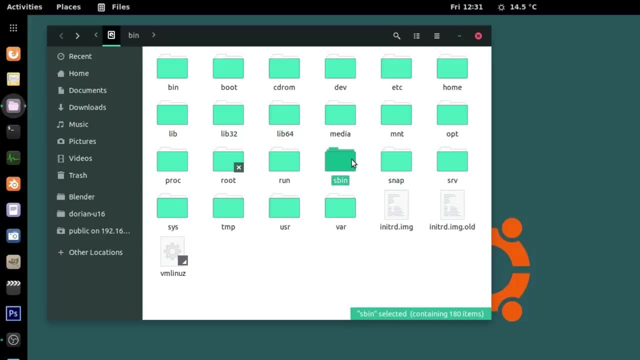 ls to list your directory, cat to display the output of a file, and other basic functions are stored here. Skipping ahead a little bit, I also want to point out sbin. These are system binaries that a system administrator would use and that a standard user wouldn't have access to without. 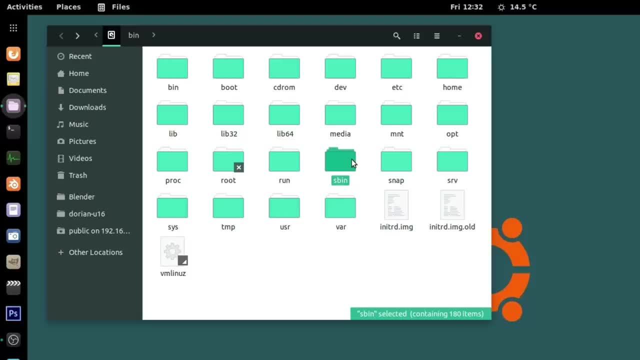 them. Both of these folders contain the files that need to be accessible when running in single user mode. as opposed to the usual multi-user mode, Single user mode is a special mode that boots you in as a root user to allow you to do system repairs and upgrades, or testing. 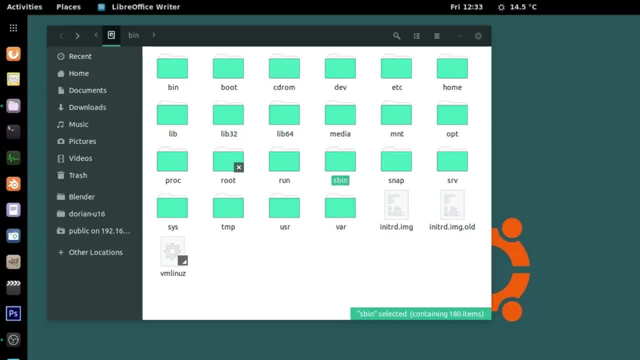 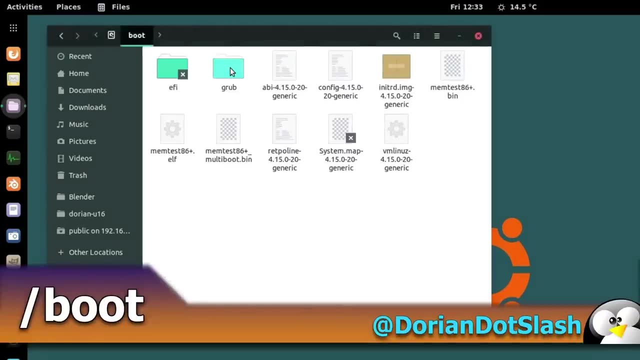 Networking is usually disabled in this mode because of security issues. When you install a program in Linux, it's typically not placed in these folders. Next is boot. This is a folder you don't want to play around in. It contains everything: your OS. 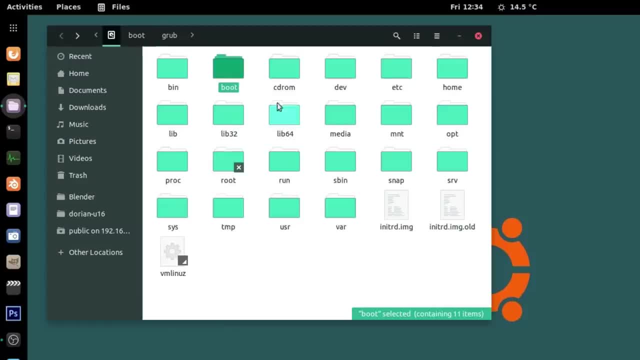 needs, including your boot. In other words, your bootloaders live here. Next we have CD-ROM, which I'm going to skip because it's not in all distros and it's more of a legacy mounting point for your CD-ROM. Let's move on to dev. This is where your devices live. 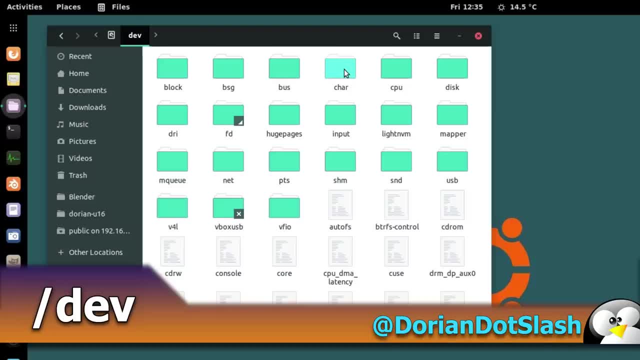 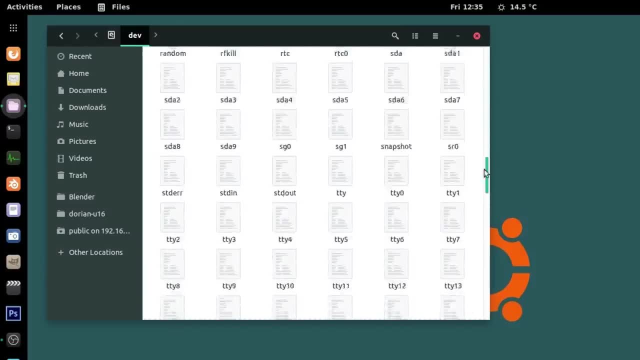 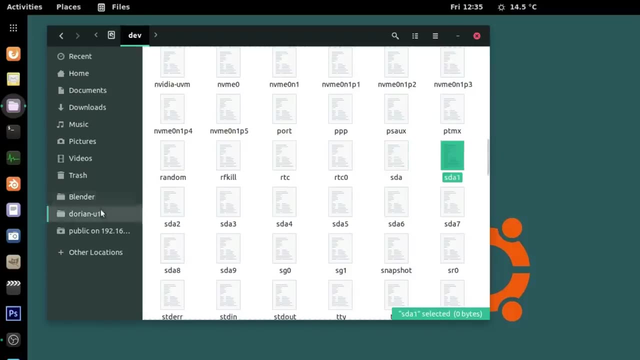 Linux, again following Unix, has a standard where it was decided: everything is a file. Here you'll find your hardware. A disk, for example, would be dev slash, sda. Here on that disk would be, for example, dev sda1, sda2 and so on. you can also find everything else here. 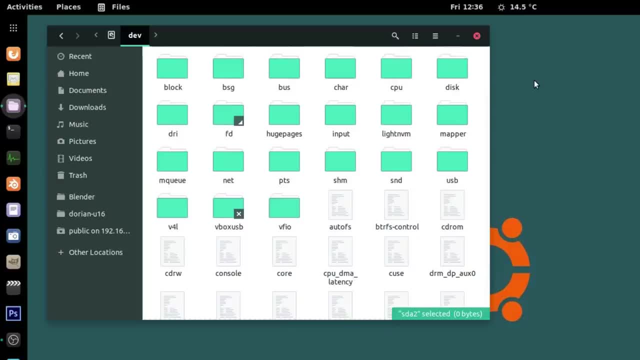 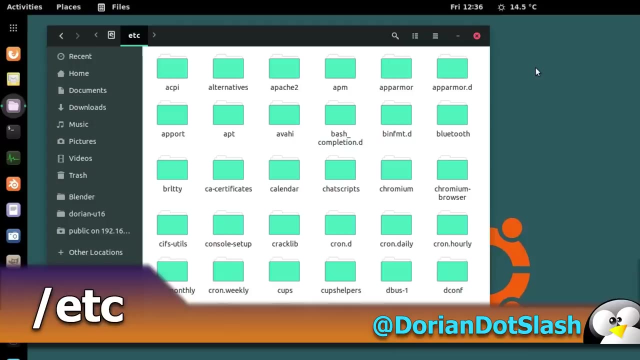 from your webcam to your keyboard. this is typically an area that applications and drivers will access and is rarely something a user should be dabbling in. so, going back to root, the next folder is etc. the name of this folder has been argued as standing for etc. edit to configure, as well as others, but it 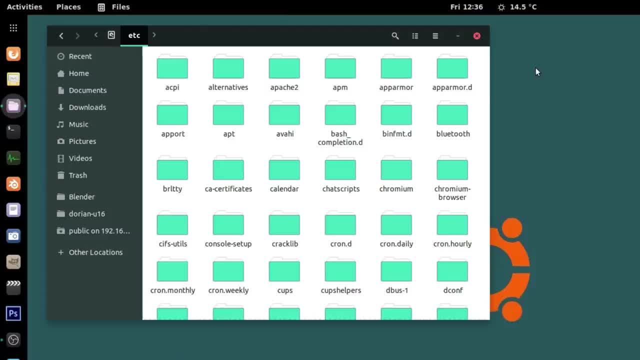 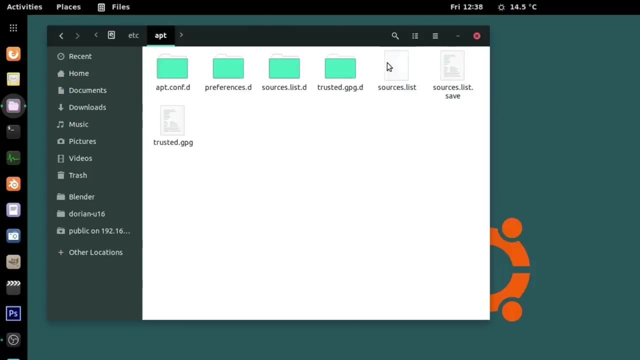 has been confirmed by dennis ritchie that it did indeed mean etc. this folder is where all your configurations are stored. however, when i'm talking about configurations, i'm talking about for things that are system-wide, such as apt. in this folder, for example, you would find the list of all your 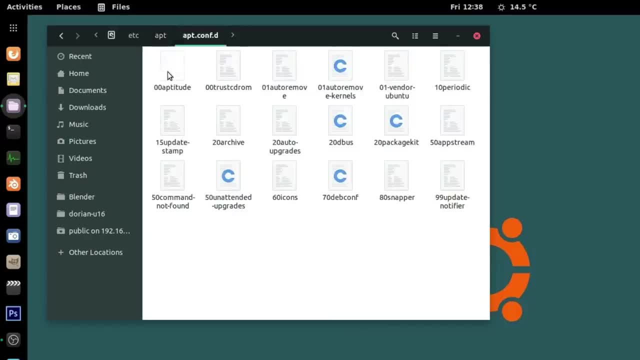 sources, what repos your system connects to, as well as its various settings. so if you're looking for something that is a system-wide application and not a per user setting, for example, if you're looking for something that is a system-wide application and not a per user setting for 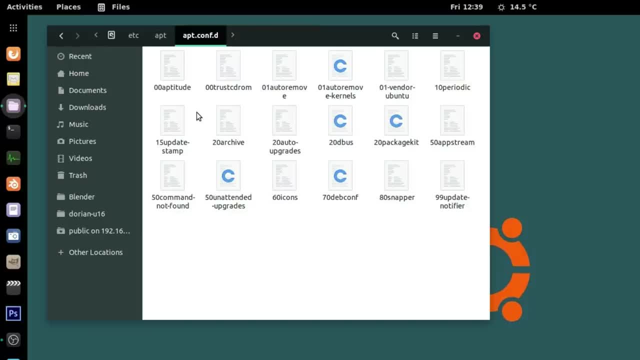 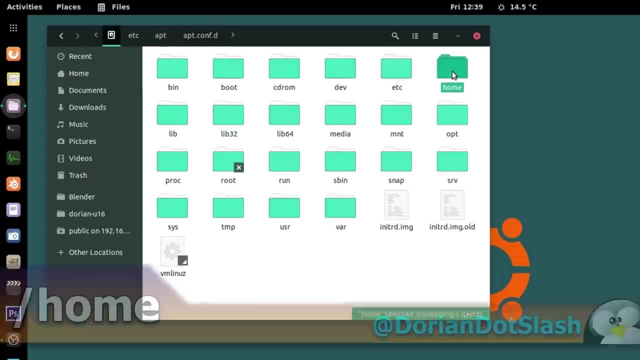 example, liber office would have settings in each user's folder and it wouldn't be system wide, because each user can have different settings. and this brings me to the next folder, which is home. however, i'm going to save this for the end, because there's some things i want to discuss about it, so we'll 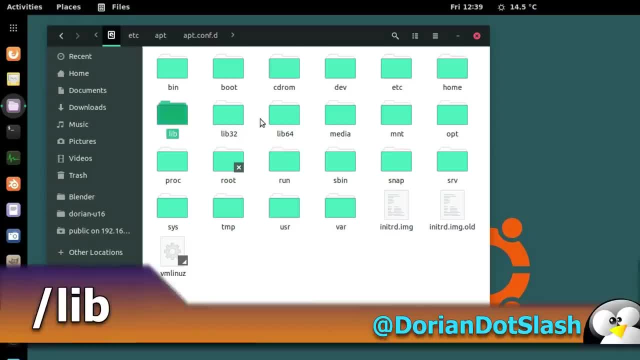 come back to it later. next are the lib folders. this includes lib, lib32 and lib64. these are where the libraries are stored. libraries are files that applications can use to perform various functions. they're required by the binaries in the library and the libraries are stored in the library. 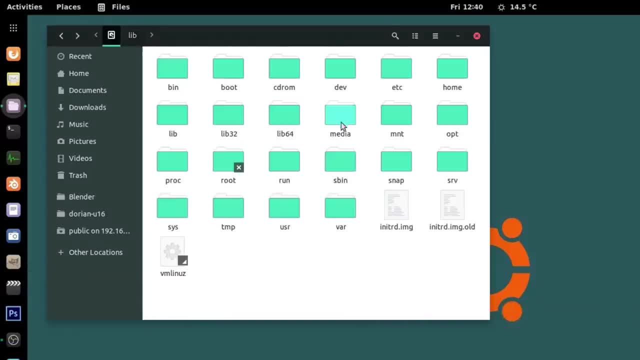 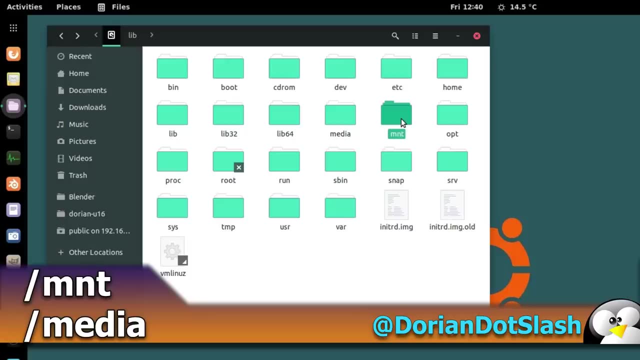 in bin and sbin, for example. Moving on, we have media and mnt or mount. These directories are where you would find your other mounted drives. It can be a floppy disk, USB stick, external hard drive, network drive or even a second hard drive. 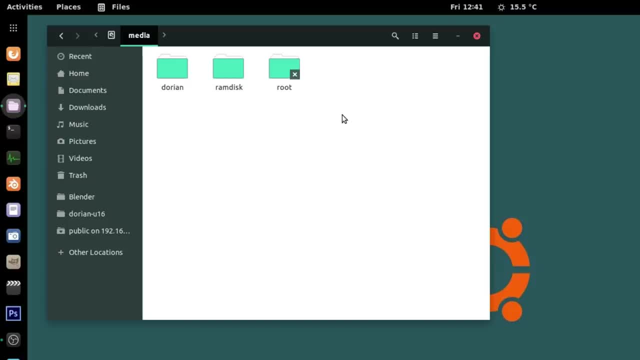 So if you're looking for that A, B or D drive, this is where you wanna be looking. Now. this media folder wasn't always around. It was typically just mnt, and that's where you mounted your storage devices. Nowadays, most distros automatically mount devices for you. 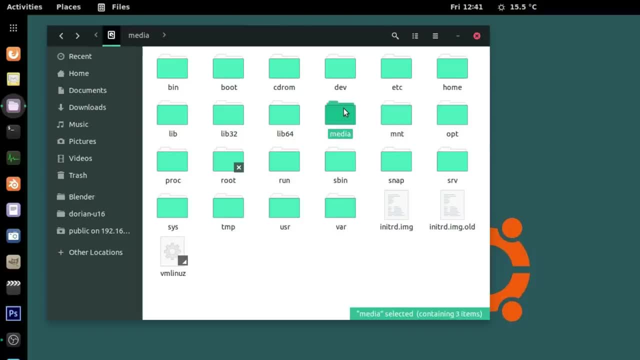 in the media directory. So your USB stick that you inserted would be in media username, device name. So why are there two directories? Well, if you're mounting things manually, use the mnt directory and leave the media directory to the OS to manage. 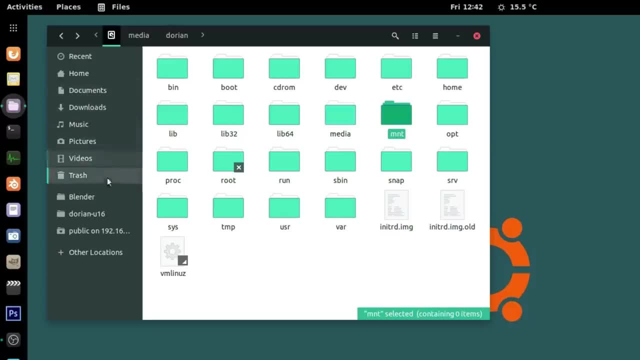 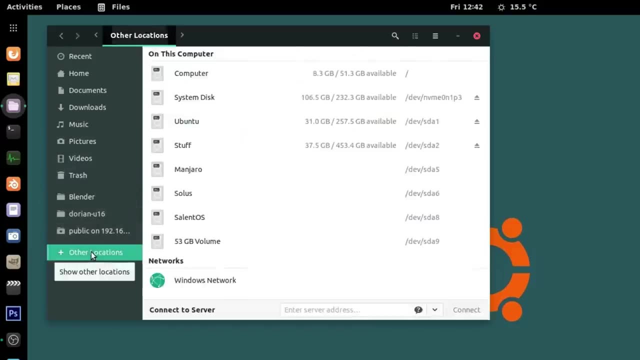 Most distros and file managers such as Nautilus, for example- what I'm using here, and Dolphin and PCManFM, will have something on the side here. For example, in Nautilus I can click Other Locations and here I can access my other devices. 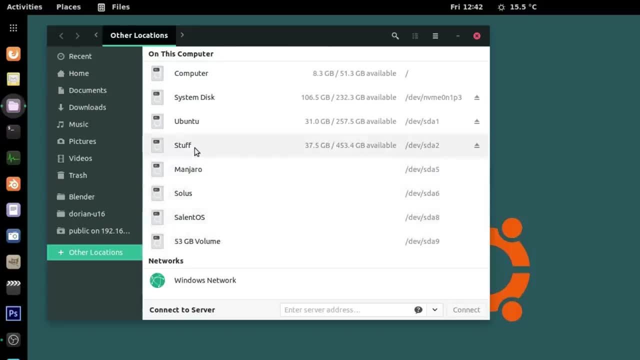 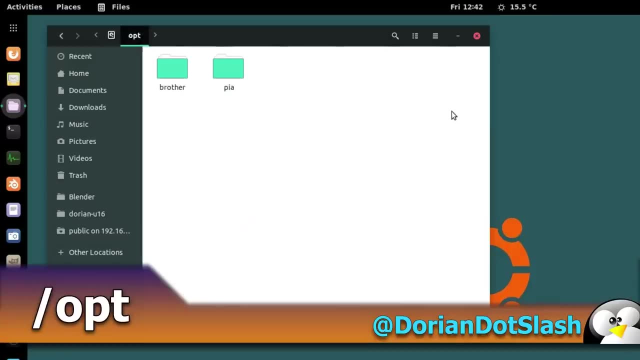 If I had a USB stick plugged in right now, it would show up here and I could simply click on it and access it. Next down the line is OPT. This is the optional folder, which is usually where manually installed software from vendors resides. 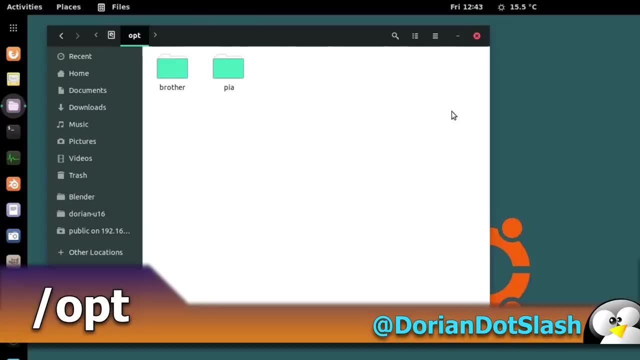 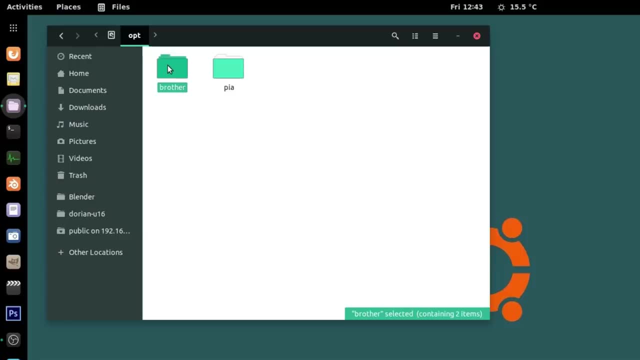 Although some software packages found in the repo can also find their way here. VirtualBox Guest Editions is one example. So here, for example, is a VPN software that I installed and the drivers for my Brother printer slash scanner. This is also where you can install software. 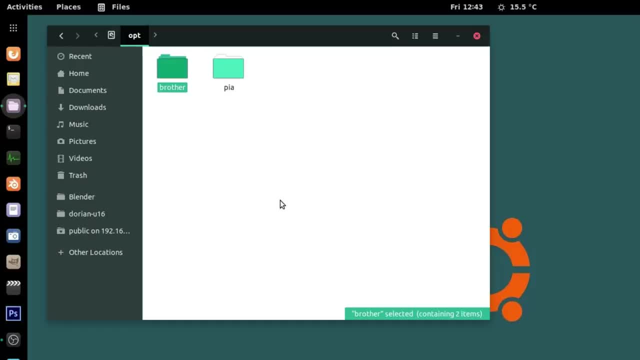 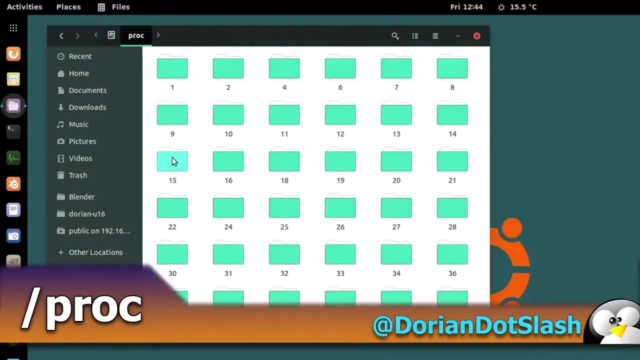 you've created yourself. This folder is where I place all the applications I've written for Scion Linux. Next we have PROC. PROC is where you'll find pseudo files that contain information about system processes and resources. For example, every process will have a directory here. 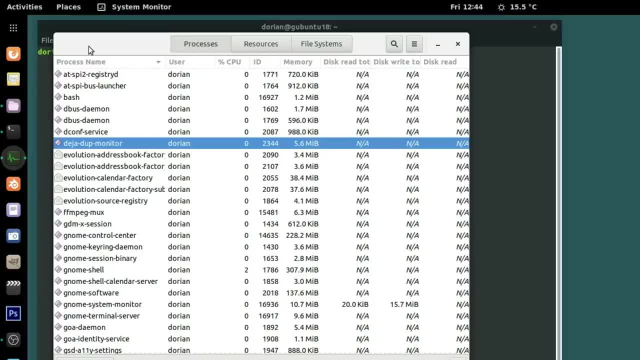 which contains all kinds of information on that process. An example I can show you here: if I open the system monitor, I can see DejaDuke monitor's process ID, or PID, is 2344.. So if I navigate to PROC. 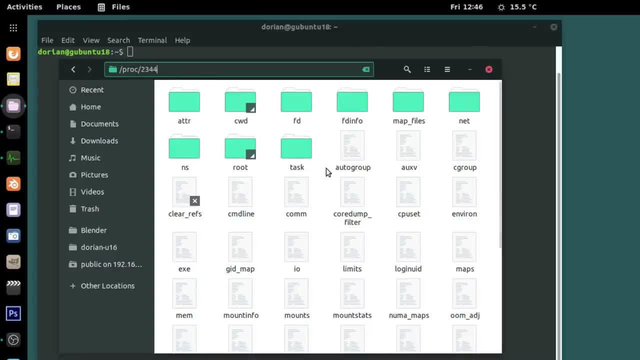 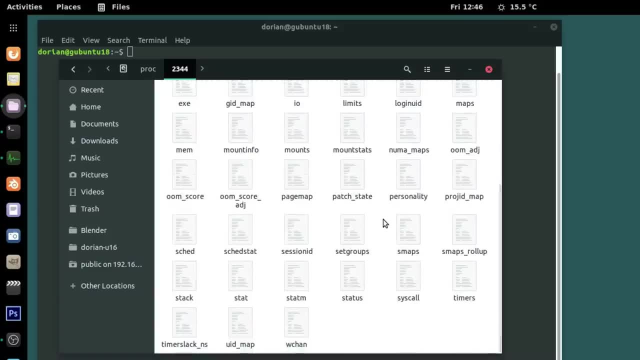 2344, which is the PID for the DejaDuke monitor. I can see all kinds of pseudo files here. This is much like dev, where they're not actually files on the system. This is the kernel translating other information to appear as files. 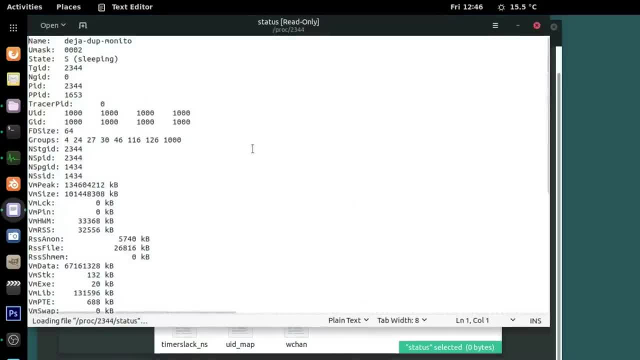 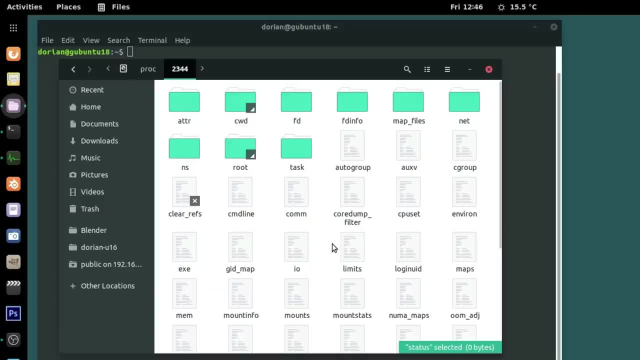 So, for example, here I can open the status file and it'll show me all kinds of information on that process. There's tons more in here, but this isn't something you wanna play in. If you are a developer, if you're writing applications, 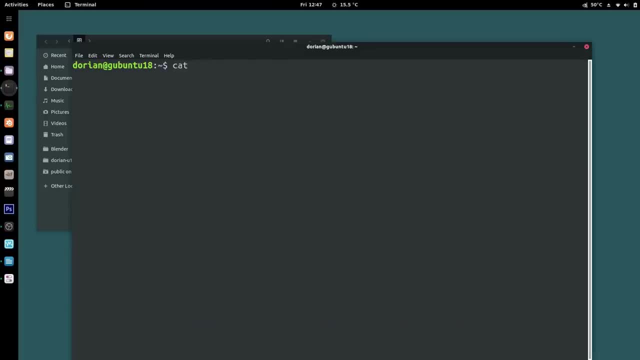 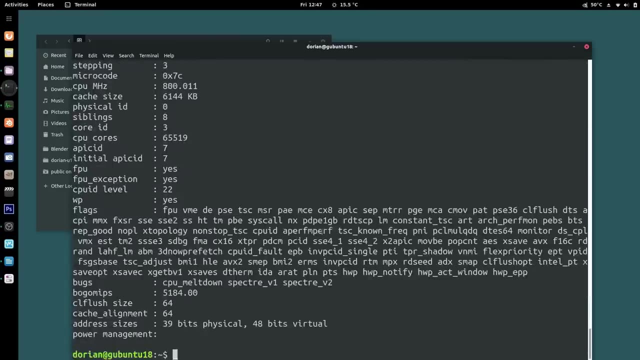 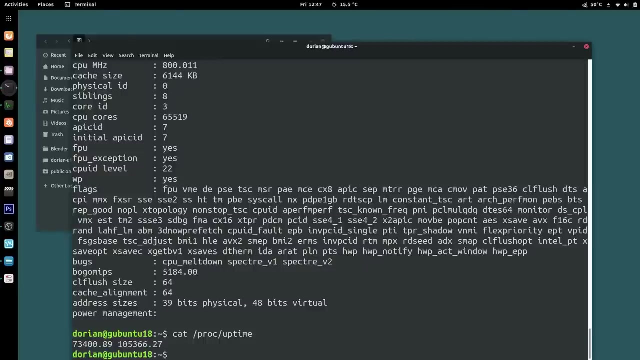 this is very handy. Here you can also find information, like for the CPU, for example. This will give you all kinds of information on the CPU and you can also do uptime, which will print out your uptime for your system. Next is root. 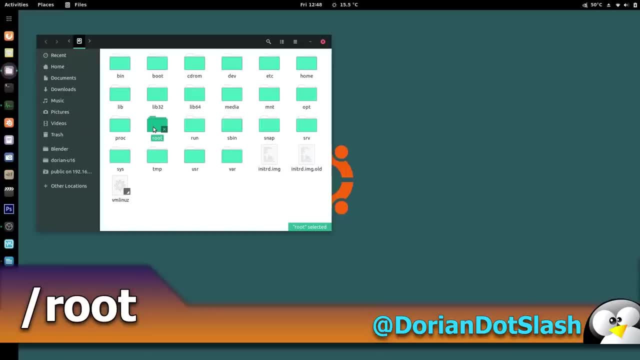 Root is the root user's home folder. Unlike a user's home folder, it does not contain the typical directories inside and it does not reside in the home directory. You can store files here if you wish, but you need root permissions to access it. 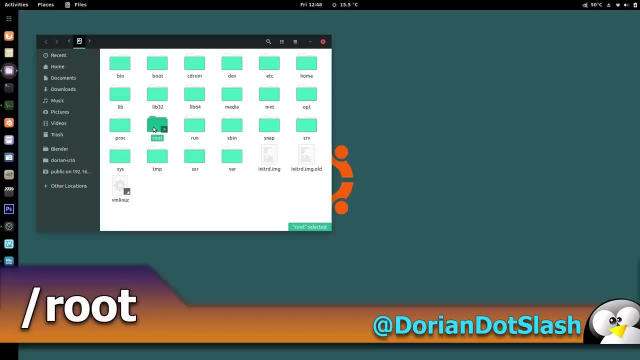 The location of this directory also ensures that root always has access to its home folder, in case you have the regular user's home directory stored on another drive which you cannot access. Next is run This one's fairly new and different distros use it in slightly different ways. 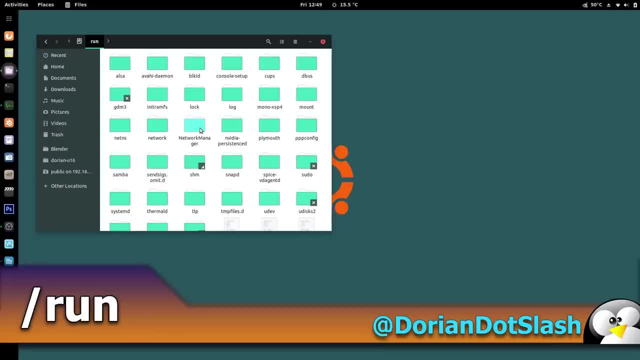 It's a tempfs file system, which means it runs in RAM. This also means that everything in it is gone when the system's rebooted or shut down. It's used for processes that start early in the boot procedure to store runtime information that they use to function. 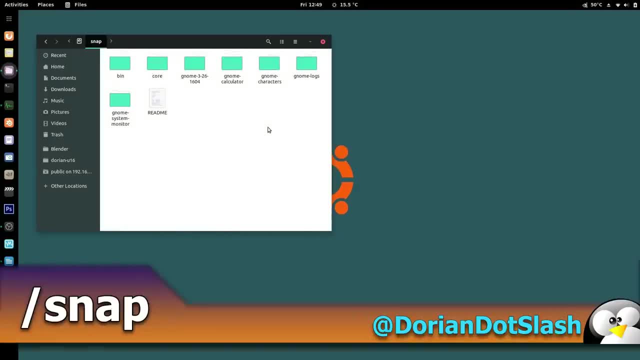 Next we covered sbin, so next down the line is snap. This is a folder where snap packages are stored and are mainly used by Ubuntu. Snap packages are completely self-contained applications that run differently than regular packages and applications. This will be covered in a future video. on its own, 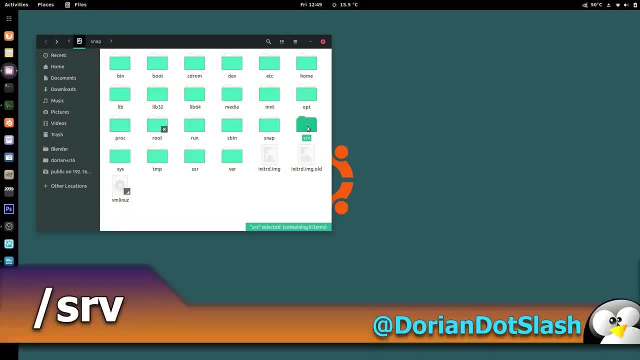 since it'll take more time to explain SRV, this is the service directory where service data is stored. It'll probably be empty for you, but if you run a server, such as a web server or FTP server, you would store the files that will be accessed. 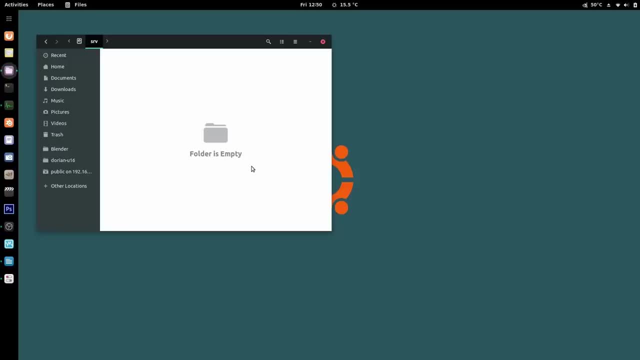 by external users here. So if you run a server, such as a web server or FTP server, you would store the files that will be accessed by external users here. This allows for better security, since it's at the root of the drive. 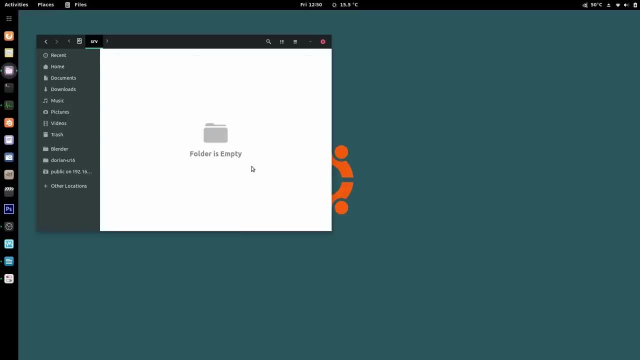 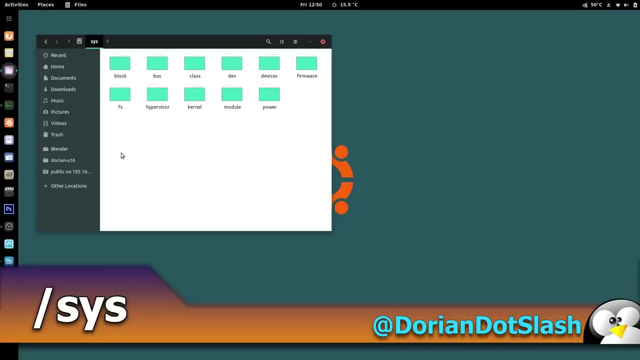 and it also allows you to easily mount this folder from another hard drive. Next down the line is sys. The system folder has been around a long time. It's a way to interact with the kernel. One older example is writing to a file using VGA switcheroo. 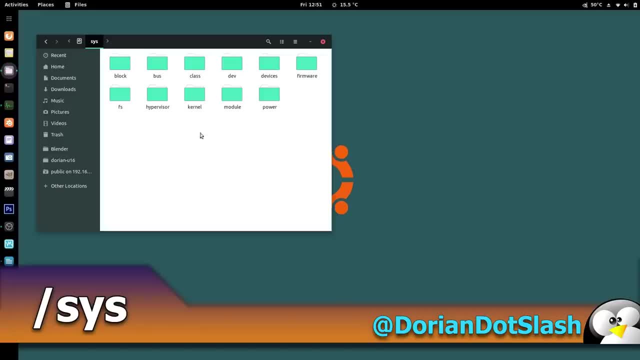 and change settings on graphic cards. in a hybrid system, This directory is similar to the run directory and is not physically written to the disk. It's created every time the system boots up, so you wouldn't store anything here and nothing gets installed. TMP is, of course, a temp or temporary directory. 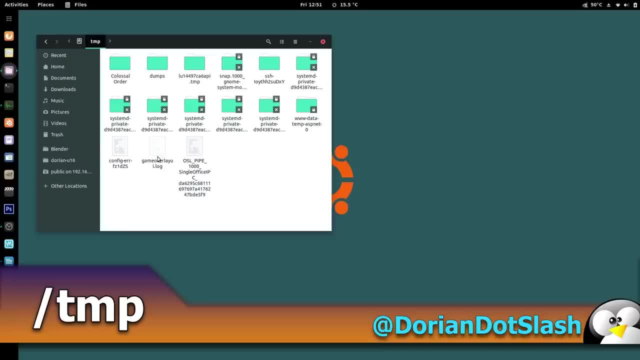 This is where files are temporarily stored by applications that could be used during a session. One example is if you're writing a document in a word processor, it will regularly save a temporary copy of what you're writing here so that if the application crashes. 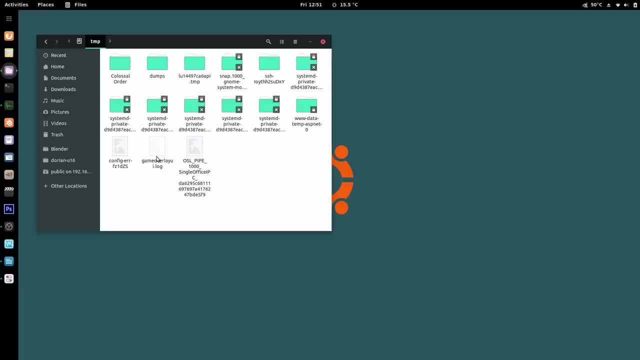 it can look here to see if there's a recent saved copy that you can recover. This folder is usually emptied when you reboot the system. On occasion you might find some files or directory that remain and could be stuck there because the system can't delete them. 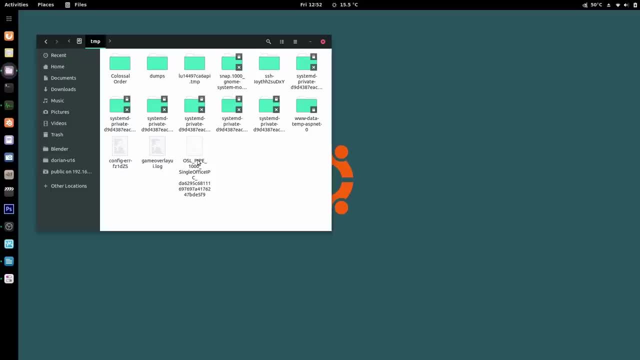 This normally isn't a big deal, unless there's hundreds of files or the files are taking a lot of disk space, in which case you might want to log in as the root user in single user mode, navigate to this folder and manually delete them. 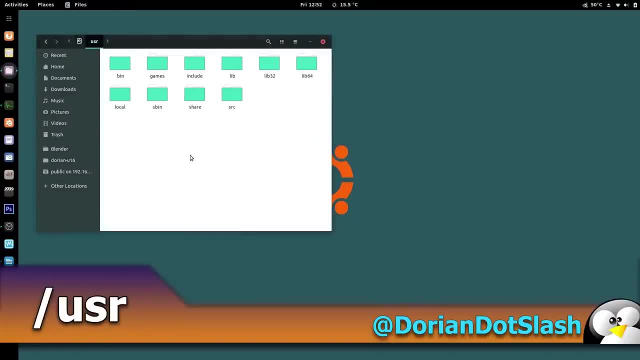 Moving on, we have the USR folder. This is the user application space where applications will be installed that are used by the user, as opposed to the bin directories used by the system and system administrator to perform maintenance. It's also known as Unix system resource. 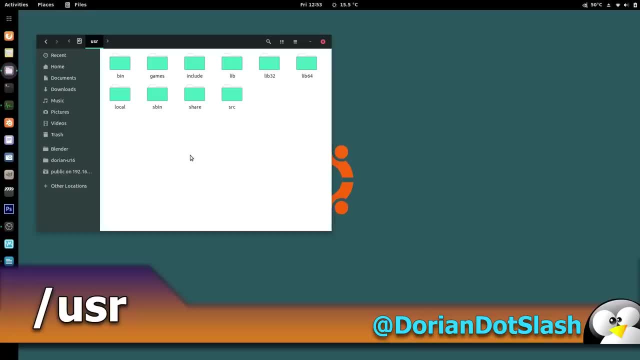 And any applications installed here are considered non-essential for basic system operation. Installed applications will reside in one of several places here, such as user bin, user sbin or local bin- local sbin- with their required library stored in user local lib or user lib. 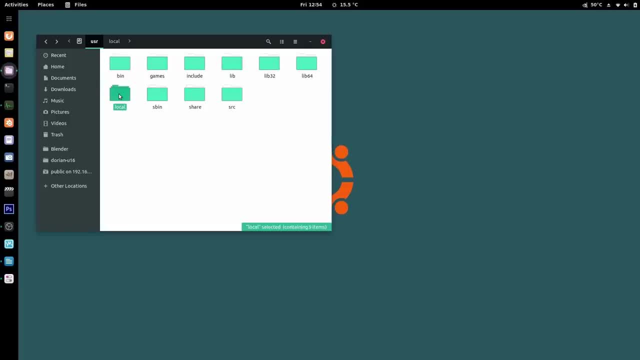 Most programs that are installed from source code will end up in the local folders. Many larger programs will install themselves into user share. Any installed source code, such as the kernel source and header files, will go into the SRC directory. This directory seems like a confusing mess at first. 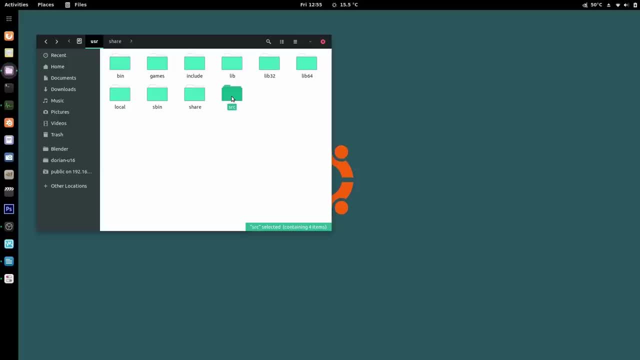 And while the directory structure and what goes where is laid out in the FHS I mentioned earlier, you'll still have to sometimes look in other places to find things. Someone making a certain application might not adhere to the standard and could just do what they want. 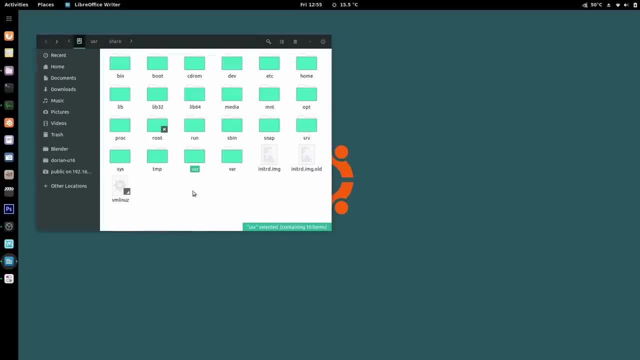 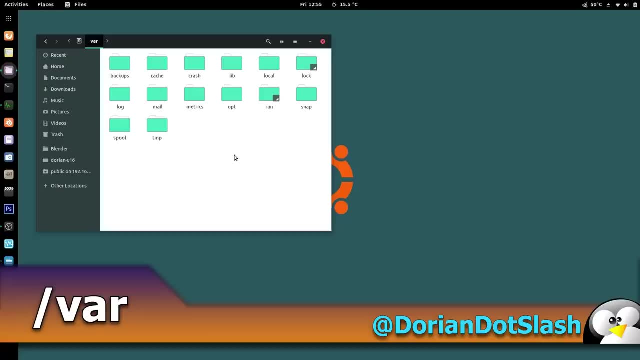 Also, some distros may treat these folders differently as well. Going back to root, we have next var. Var is the variable directory. It contains files and directories that are expected to grow in size. For example, var crash holds information about processes that have crashed. 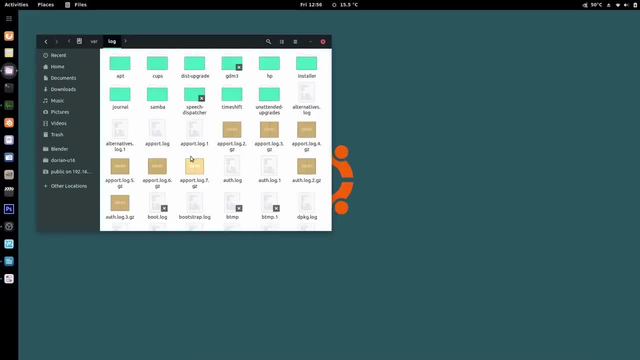 Var log contains log files for both the system and many different applications, which will constantly grow in size as you use the system. You'll also find other things in here, like databases for mail and temporary storage for printer queues, also known as the spool. 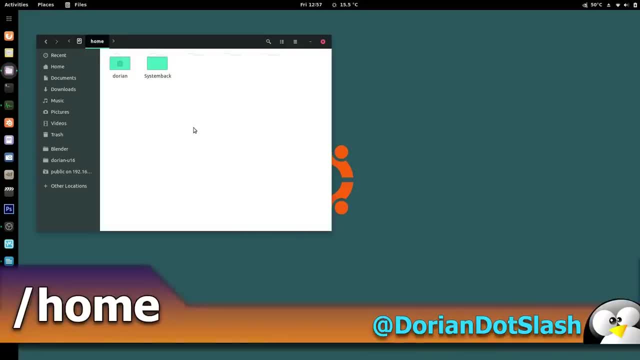 And finally, we will come back to the home folder. When you enter the home folder, you'll see a list of files. You'll see that each user has its own folder inside of it. The home folder is where you store your personal files. 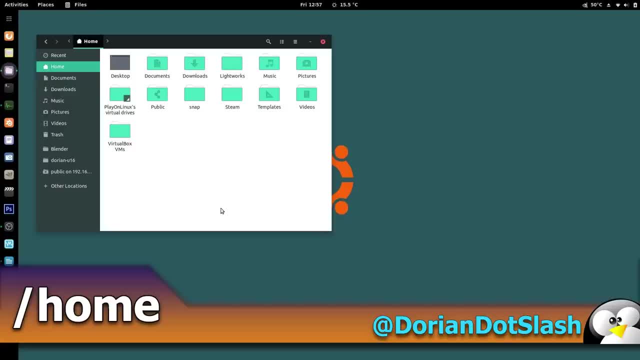 and documents. Like I said, each user has their own home folder and each user can only access their own unless they use admin permissions. Some users mount the home folder on a different drive or different partition, which allows you to reinstall your system and preserve your files. 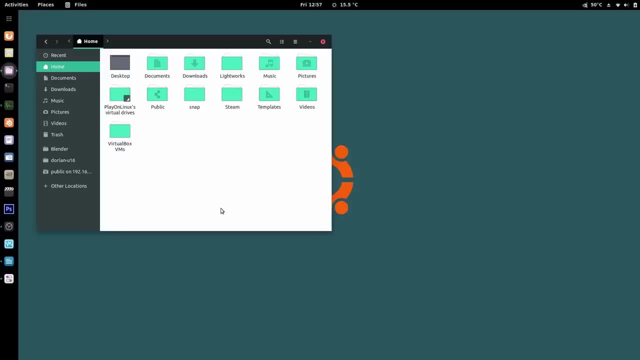 The home folder also contains many different directories which store your application settings. A hidden directory is simply one that starts with a period. Linux hides these by default. You can view them in the file manager by selecting Show Hidden Files or by pressing Control-H. 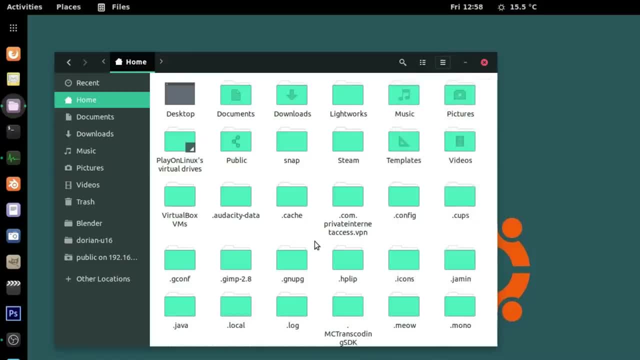 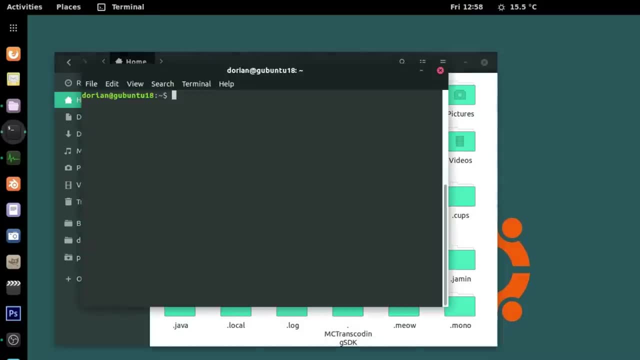 This is, of course, using Nautilus in GNOME and some file managers might be different. PCManFM is also press Control-H to view hidden files. If you're in the terminal and you list files, it'll only show you what is not hidden. 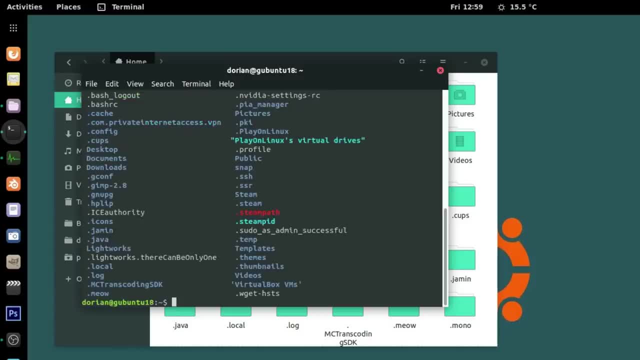 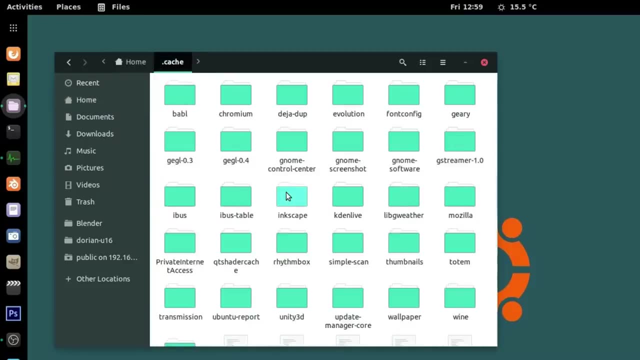 unless you specify dash A for all. And now you can see all your hidden files. These hidden directories store things like cache that some applications, like a browser, use to store temporary files. Other applications might store thumbnails or information that will be used over and over repeatedly. 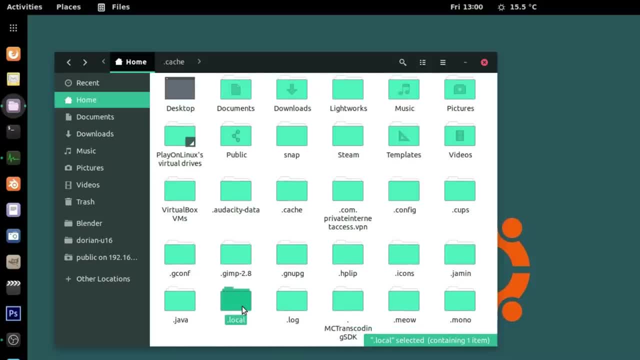 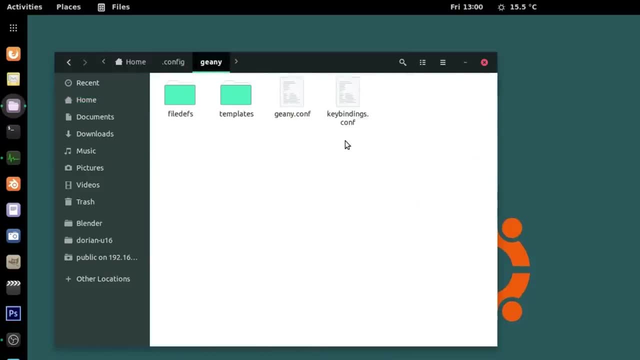 Then you have folders like config and local, which store individual application settings. Genie, for example, can be found in config. So here's the Genie folder. Any settings that I change in the Genie options are saved here. If I go back to the home folder, you 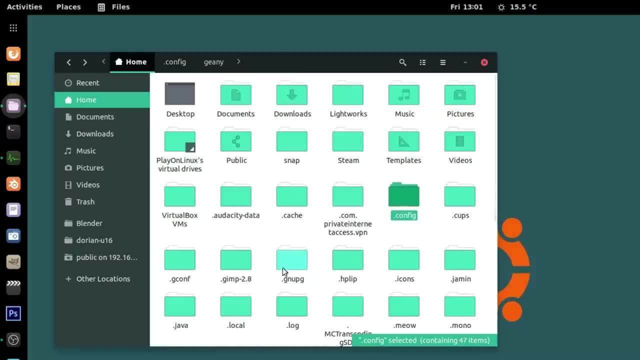 can see that some applications store their settings straight into the home folder, like GIMP, for example. These hidden folders are also where your desktop settings are saved. Whether you use Openbox, KDE, GNOME, Unity, they all save their settings here. 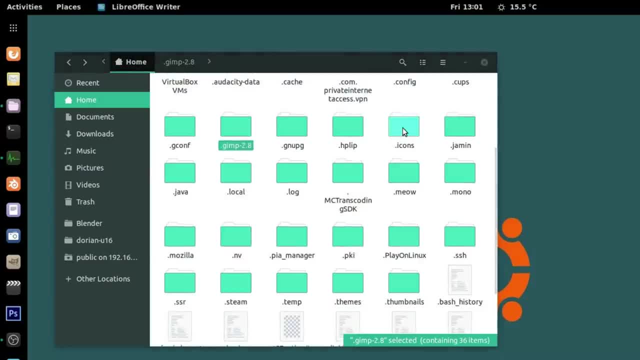 such as what wallpaper you use, what theme you use, and so on. You could even place your icons and themes in these folders so that you can have a custom look and easily save them for reuse. These hidden folders are important if you want to back up your files and your settings. 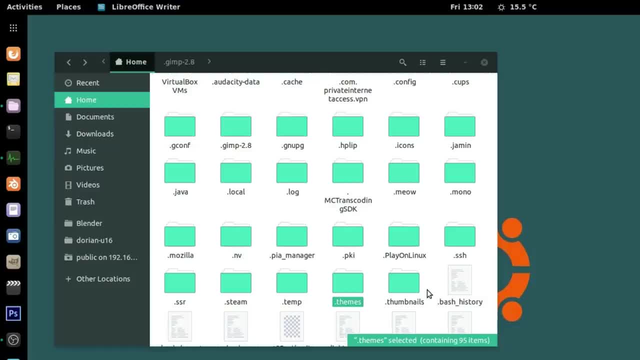 I covered backups- how to do them and where to store them- in another video, which I'll link in the corner of the screen It's in the description below. If you don't customize your system or you don't care to, then you can simply back up all the folders you see here. 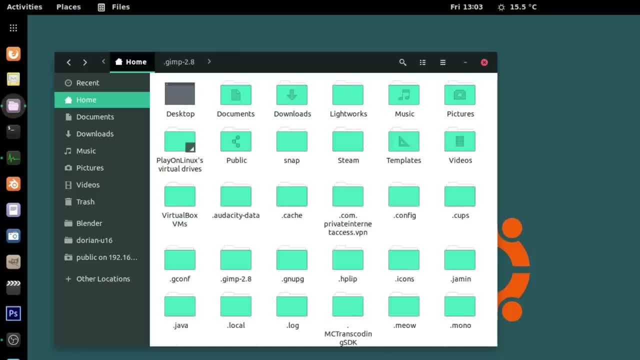 If you want to save all your settings, then you might want to include all the hidden files as well. So if you reinstall your system, you simply log in and all your theming will already be done, just like you left it. You will have to reinstall your applications. 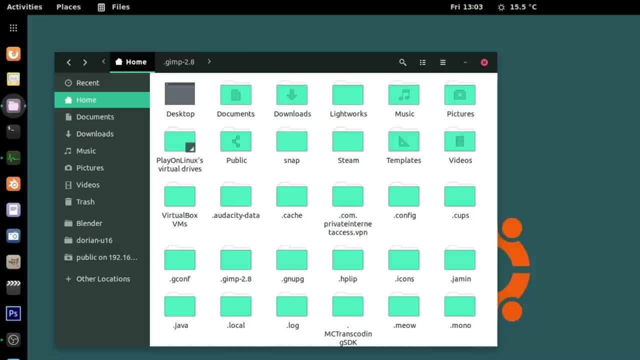 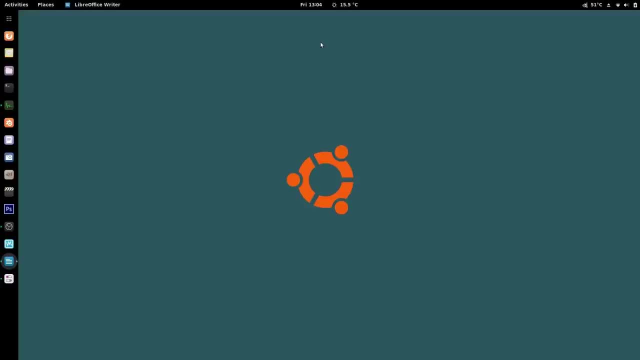 but once you install them, the settings you set for them will already be in place and the applications will run just like they did before. So, as you can see, Linux is kind of similar to Mac, but very different from Windows. Although it seems like a mess, it's actually. 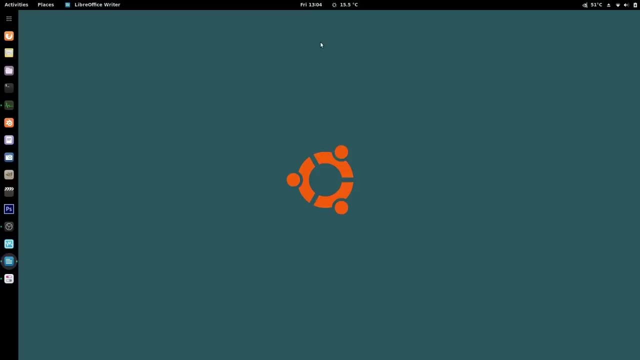 a more efficient way of doing things and allows much more sharing of common resources between packages. When it comes to adding and removing software, your distro will have a package manager that will handle all this for you. Package manager tracks where everything is going.